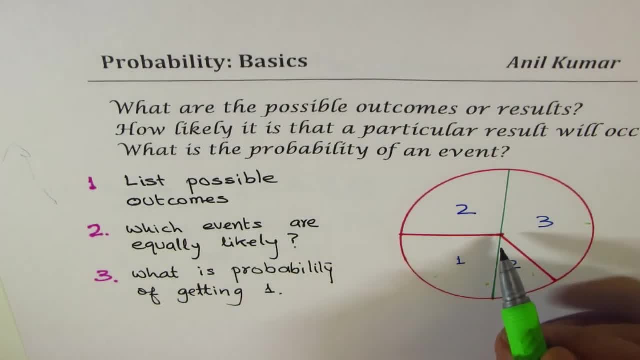 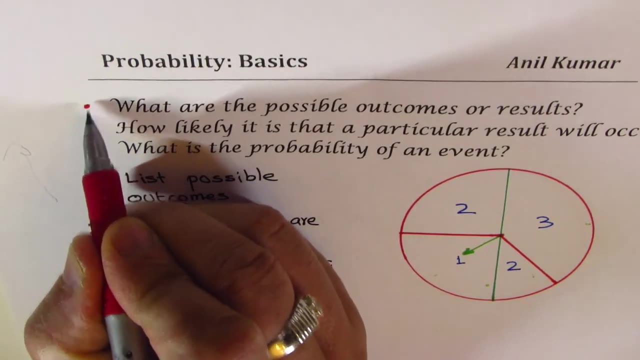 So in a spinner you have a circle, some numbers written and there could be a pointer right. So they could be a pointer, which I've just made here. Now we'll actually concentrate on three types of questions. The first one is: what are the possible outcomes or results? So, whenever 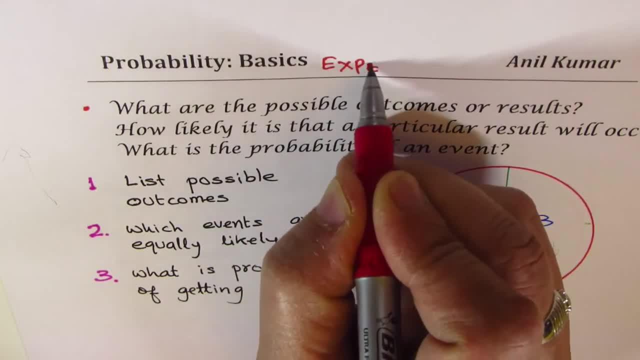 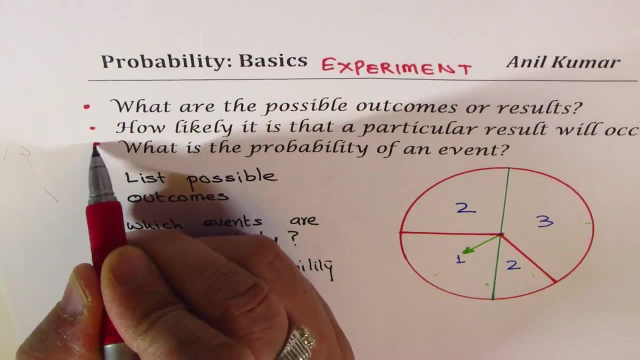 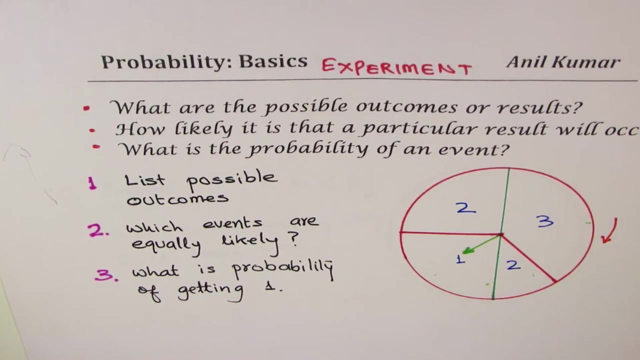 you perform an experiment, in that case there are some outcomes and results. So that is what we mean Now here. the experiment is to spend the spinner, right? so that is what the experiment is. so when you spin, where will this pointer be? those pos, those are the possible outcomes, right? second question will be: how likely? 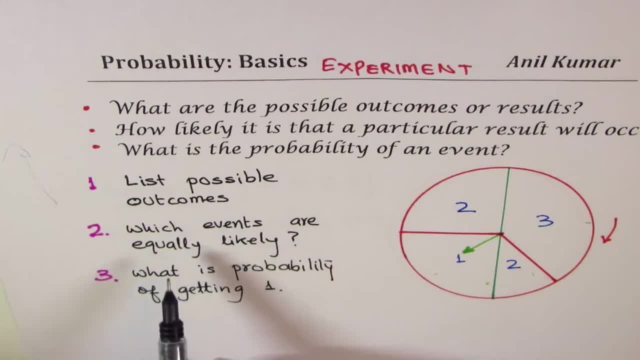 it is that a particular result will occur. so we'll specify what we are looking for, and then the third question will be: what is the probability of an event? now, probability is favorable outcomes to total number of outcomes, correct? so that is how we will be answering these questions. 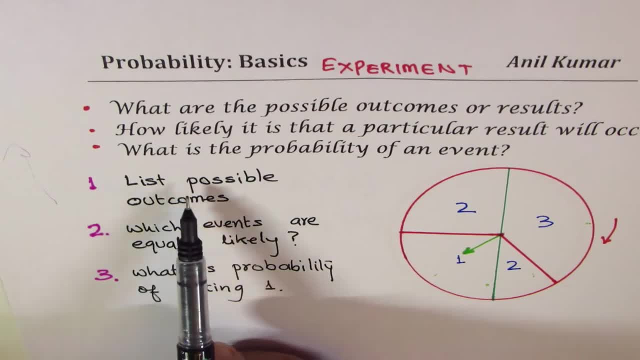 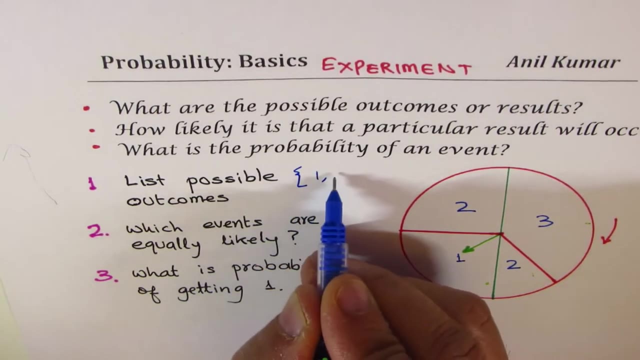 now let's begin. the very first question is list possible outcomes. now, in this particular spinner which you see, what are the possible outcomes? the numbers one, two and three are the possible outcomes. these are written in curly brackets so we can write them as one, two and three. 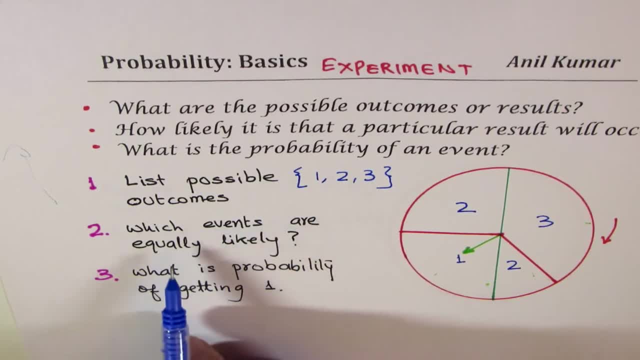 the second one is which events are equally likely. equally likely means they have the same chances, right, so they occupy the same area in case of spinner. so you can think about area when you work with spinners. okay, so which are the two equally likely events? now you will see that one is small, so that will not work. then two, so this particular 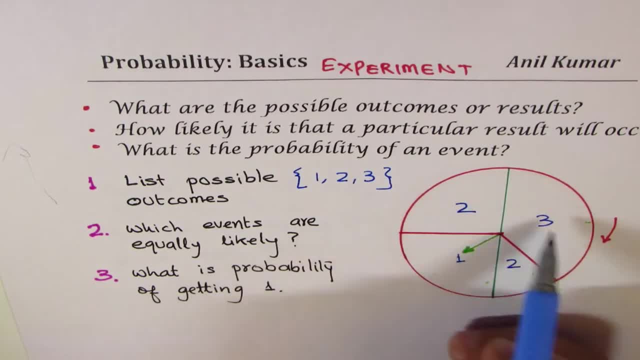 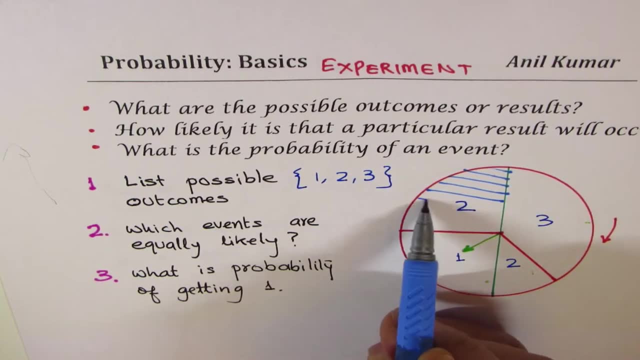 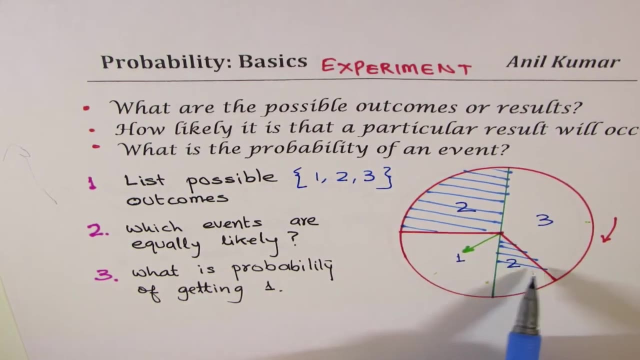 event is the two equally likely events. so you can say that this is quarter, this is one, eighth, you will notice that two and three are equally likely. see, if i shade, then you can make out that this is two. right, this is two, this is also two. so so if you combine these twos, then 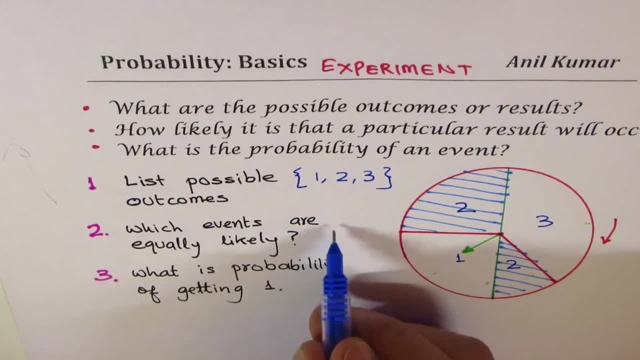 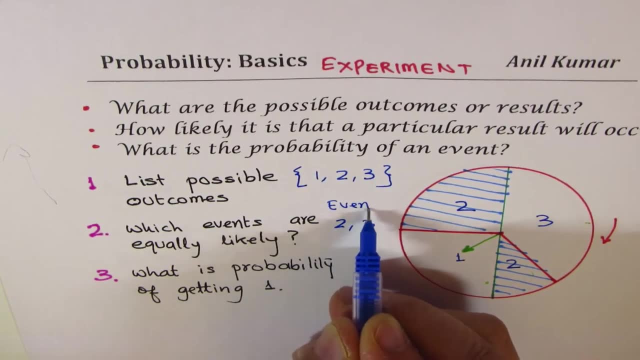 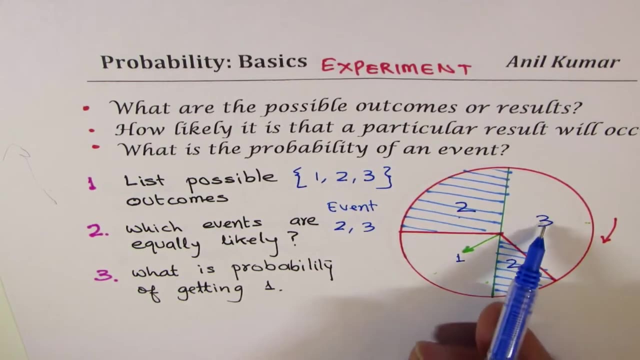 three and two area is very close, correct. so we can say getting two or three right, so that event event of getting two or three are equally likely. i hope that's clear right. since the area of two and three is same, what is the probability of getting one? 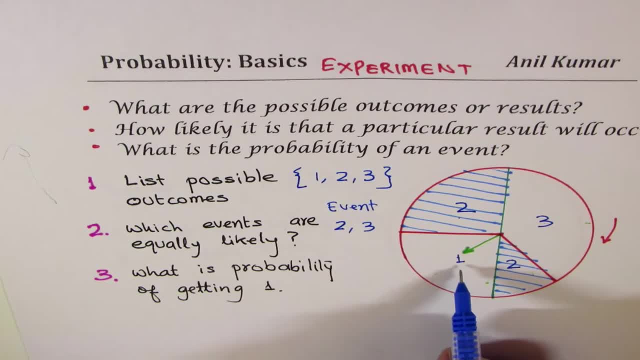 now, if i see the whole, one occupies only one quarter of the place, right? so this probability is one out of four, correct? so probability is always a fraction, which is at the most one. so it is between zero and one right, both included. so in this particular case, one occupies one fourth of the 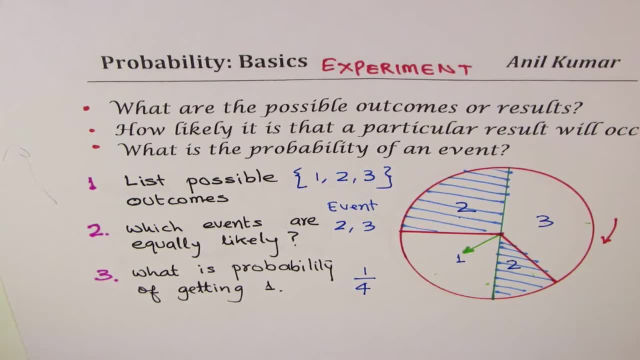 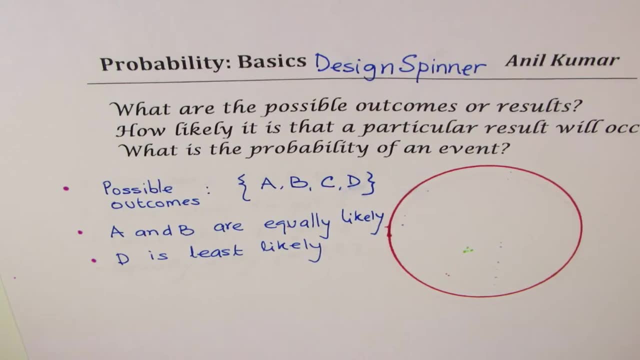 area. so it will be one out of four, perfect. now let's see other questions related to spinner in this video. the second question here is you, again the same thing. we need to find what are the possible outcomes, how likely it is that a particular result will occur and what is the probability of an event. however, this time we 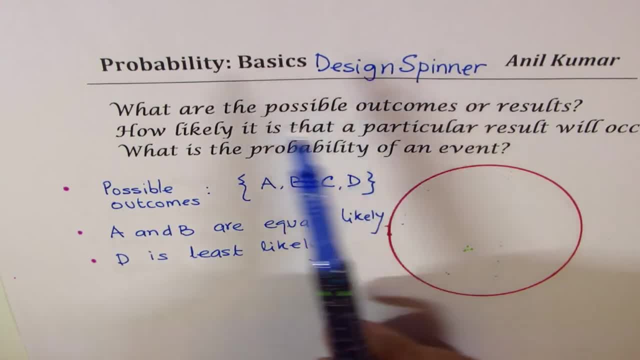 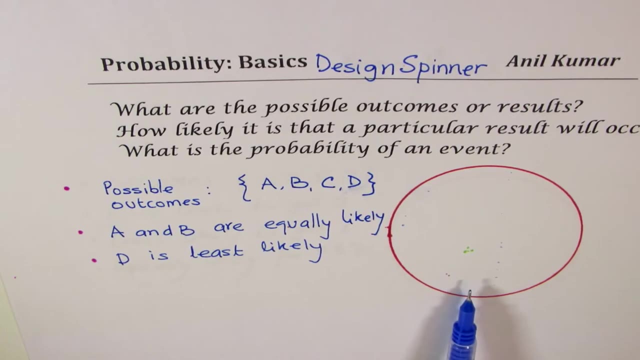 are doing different thing. we are designing a spinner. so the idea is to design spinner which could do all this, that is to say, a spinner whose possible outcomes are a, b, c and d. that means we have to divide it into four parts and a, b, c, d will be allocated to those parts. then second thing is: a and b are equally. 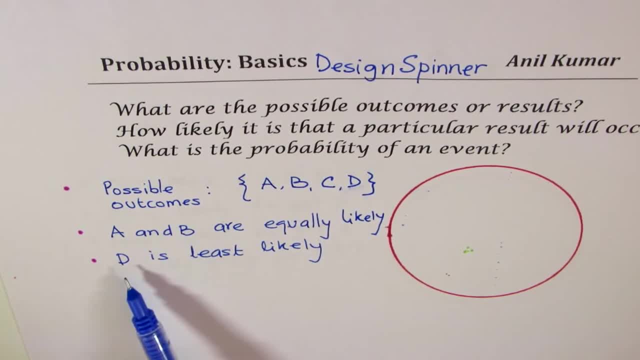 likely. so a and b are equally likely. and then we are also given a condition: d is least likely, right? so that is what it is now. it can have many solutions, right? so first thing is that we want to make a and b as equally likely. so let me focus my attention on holy s finding the hundredths. in this particular case and guess where we are at. so in the first, very first member, i'm, and its now that we are likeeyed. so now arraign our eyes on this one because of let me do this, so that way we will determine the possible outcomes. so, while i focus my attention on all, teach on any. it can also. 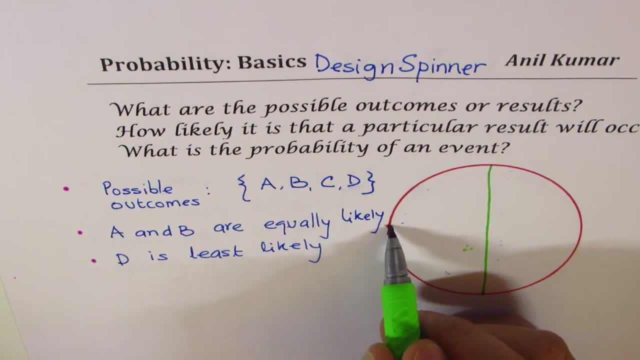 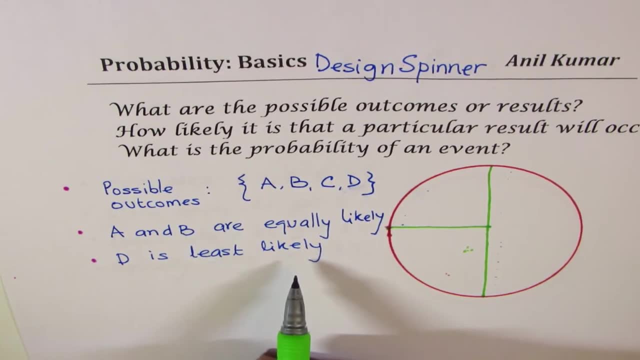 first divide it into half and let's say: let's do like this, but we want D to be least likely. you understand, D is least likely and A and B are equally likely. so what can you do? so what we can do here is that we can divide a quarter into two equal parts, for example. right, so let us say this: 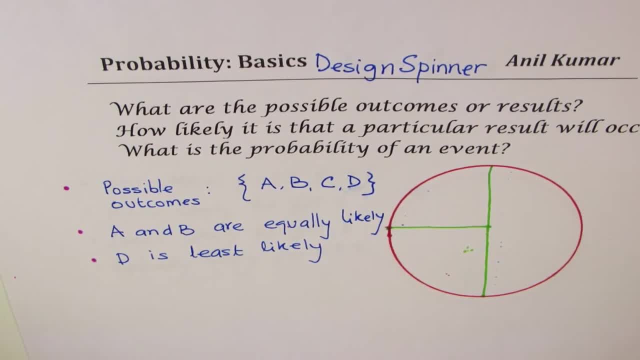 is, this is one quarter, so I'm going to divide this into two equal parts and write A and B in those parts. so this becomes A, this becomes B. as you can see, A and B are equally likely. perfect, now we have to make D as least likely, so let me reduce this area further, right? so let me say: 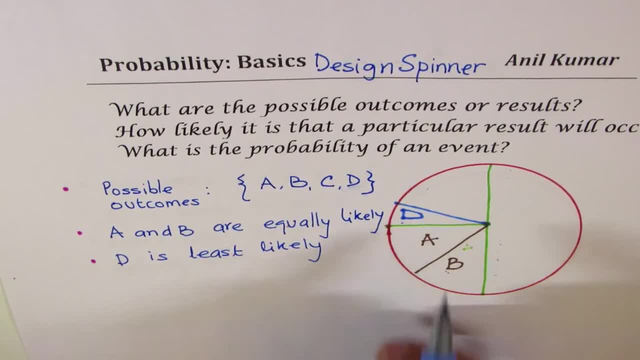 this much, only so let me reduce this area further. so let me say this much only: I'm writing D here, so D is now least likely perfect, since the outcomes are only for A, B, C and D. so all this rest area I can mark as C. you get an idea, so that becomes a spinner where C is most. 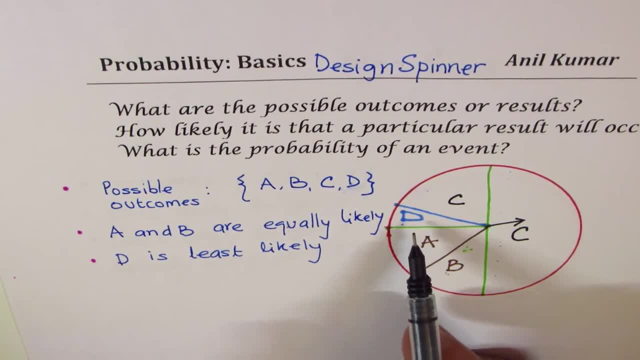 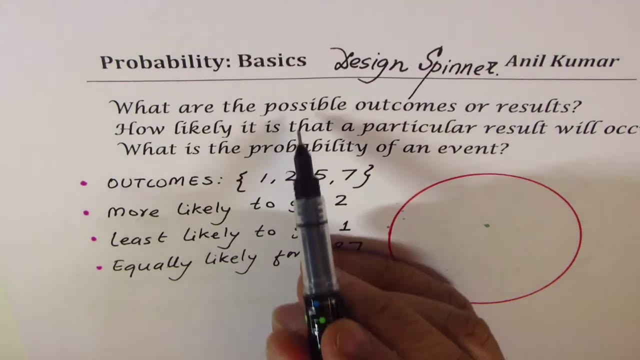 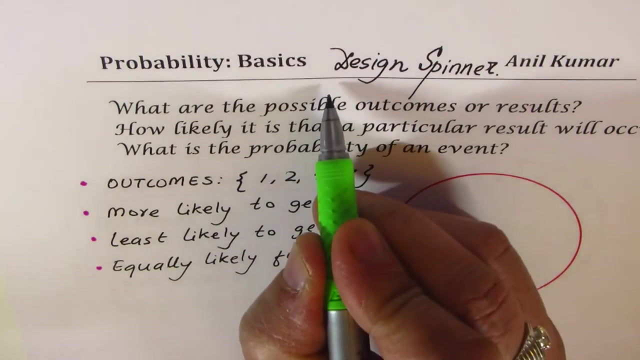 likely. A and B are equally likely and D is least likely. so I hope that makes sense. so like this, you can design your own spinner, perfect. next question is for you now. these things, you know, are same. this is what we want to understand. but again, we are going to design a spinner now, so again, you have to design. 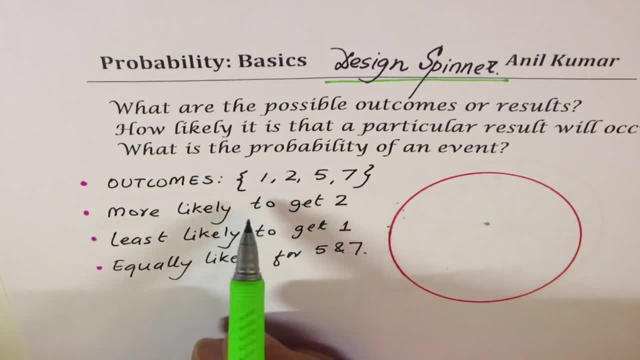 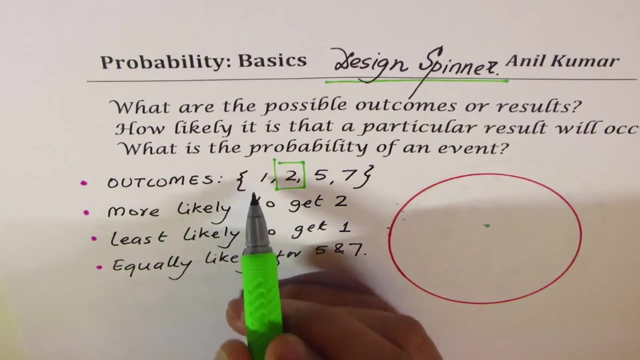 a spinner this time. the conditions are that the outcomes are one, two, five and seven. there are four outcomes with these numbers. more likely to get two, so this is more likely. so it's a big one. least likely is one, so this is very, very less, very, very thin. equally likely are five and seven. so 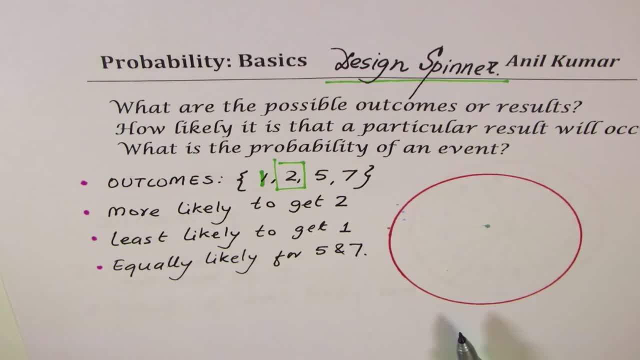 similar to previous one. I would like you to pause the video, copy this question, solve and then look into my solution. right so you, there could be many solutions, as I said. so again, what you could do is it's always good to divide it into two parts first, and preferably two equal parts, and then you can. 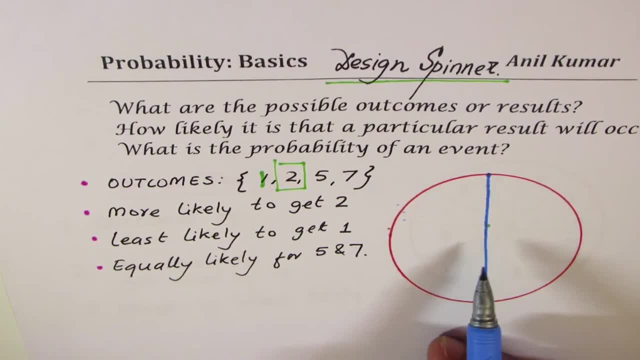 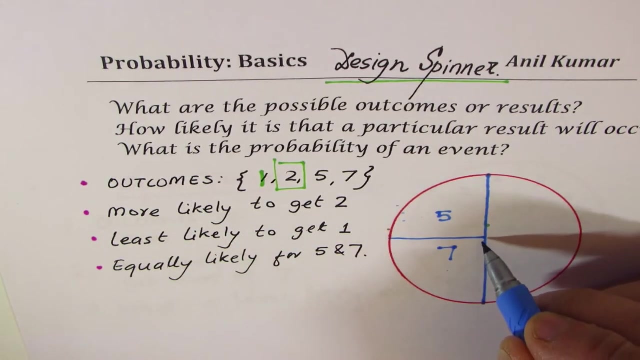 do it in a bigger way so that it is two parts correct. so we get two parts. now we want to make least likely for one equally likely for five and seven, right. so you can do like this: so we have five and seven as equally likely, right, least likely for one and more likely for two. so we can just 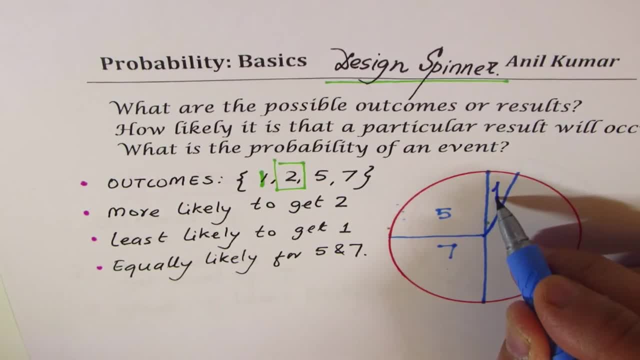 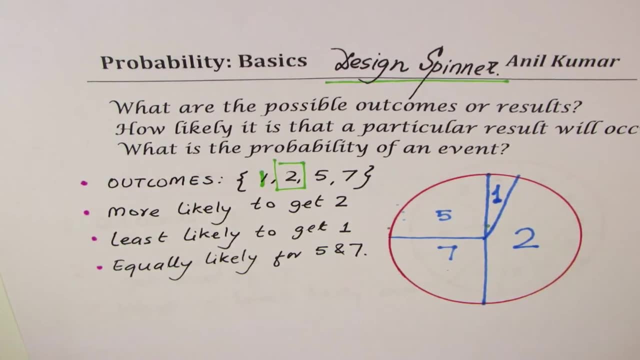 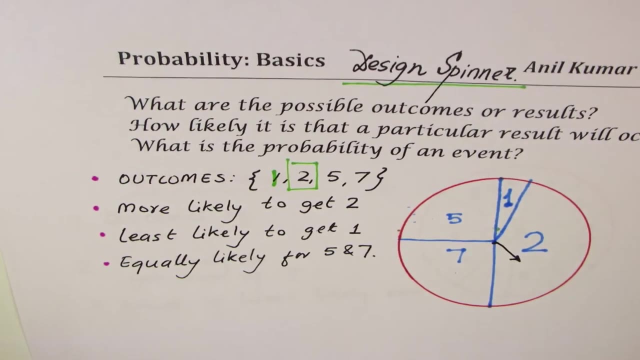 take away a small slice from here for one and leave the rest for two. so this is just a small. do you see that? so it is a very easy way to make a spinner from the given conditions. do you agree with me, right? so, and that becomes the pointer, right? so? that is how we can always. 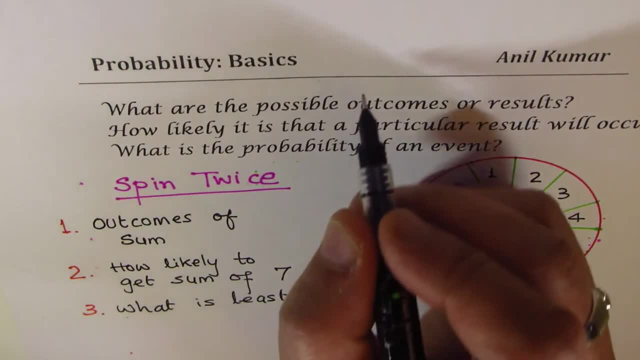 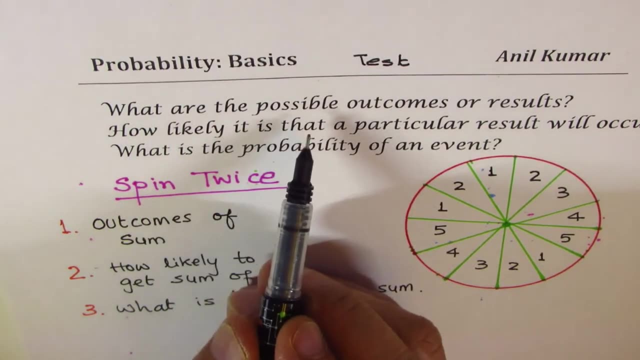 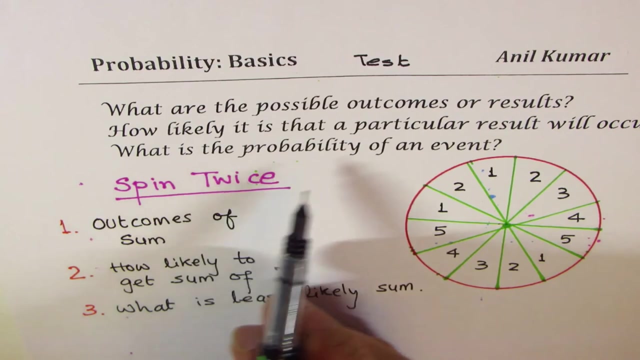 design a spinner. now here is a test question for you. this is slightly more difficult now. in this case we'll again look for possible outcomes or results and how likely it is that a particular result will occur and what is the probability of an event now in this particular. 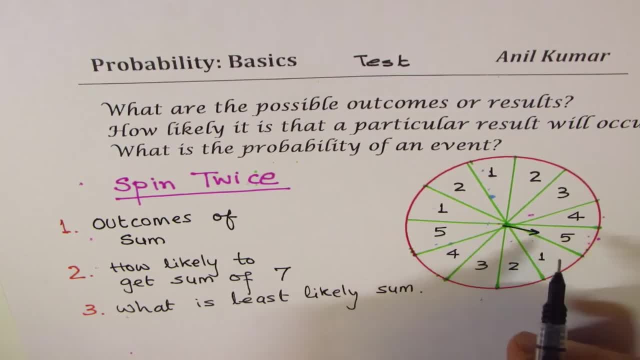 case, we are going to spin this spinner twice. spin twice and then write the outcomes of sum. so the numbers are from one to five. if you spin it twice, what sums can you get? you have to write those sums. how likely to get sum of seven, what is least likely sum? 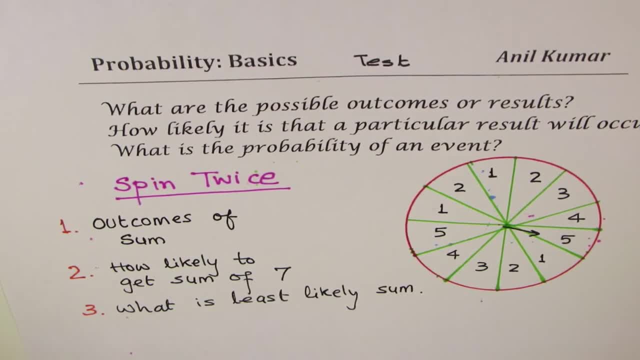 so that is what you have to answer: perfect. so let us concentrate on finding the sum first. so if i spin it twice, it could land at five and then again at five. so 10 will be the highest number. it could land at one and again one. two will be the lowest. so i have all the numbers from 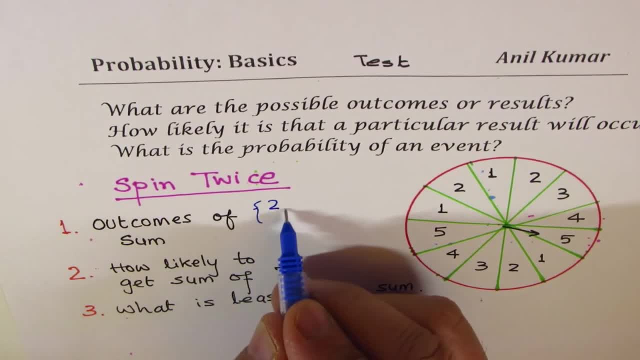 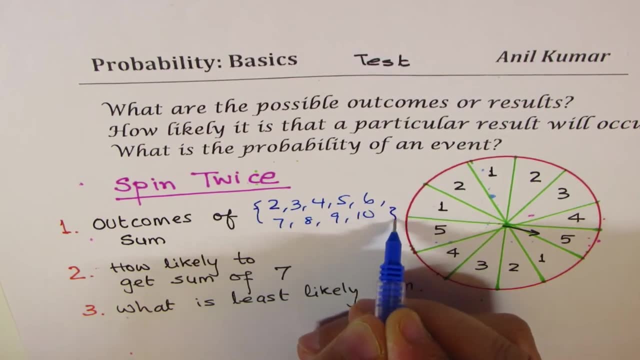 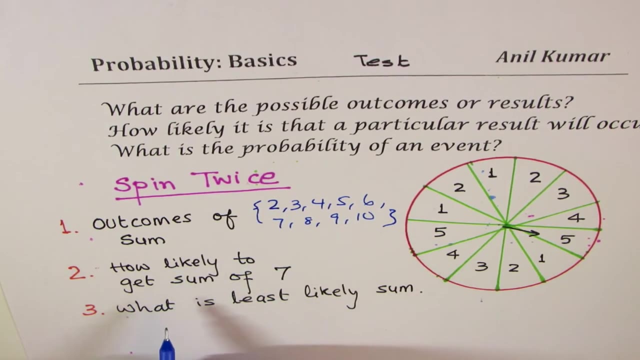 two to ten. i hope you agree with me right? so so we get two, three, four, five, six, seven, eight, nine and ten as the possible outcomes. so these are all the outcomes which we are expecting. now the question is how likely to get the sum of seven. now, how do you get seven? well, there are. 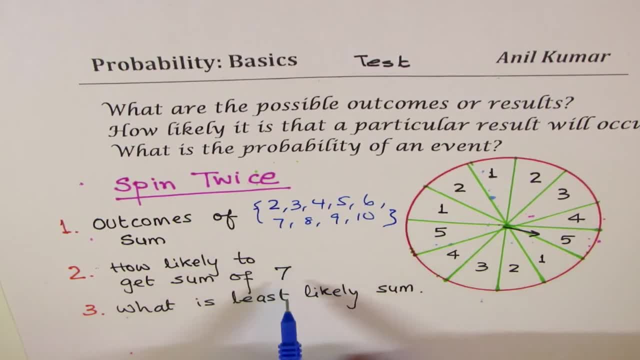 10 ways of getting up to 10. so there are all these numbers, but you, you to get seven. how many times can we get seven? we could add two and five, three and four, right? so those combinations will get seven to you, right? so seven is like two plus five is seven, or it could. 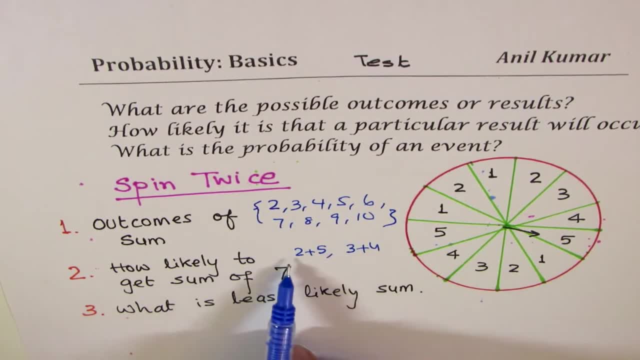 be three plus four right or four plus three right, so that is how you could get seven. so get getting seven. so it's more of a combination of high number one two. this is something we don't like to do, right, so we don't have many combinations right. so so more or less you can say it is less likely. 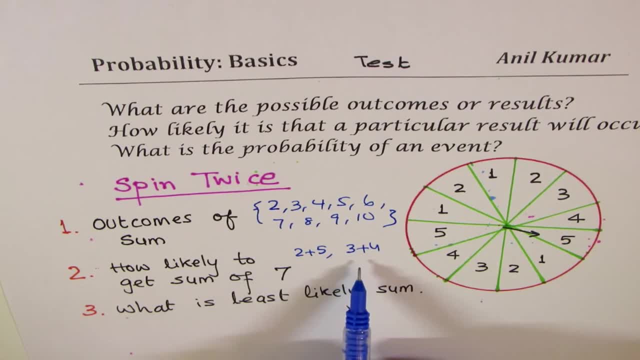 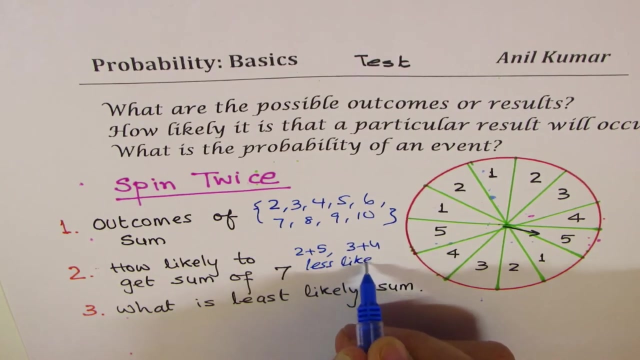 right, it is less likely, right? so that could be one of the answers for us. now, i think you can get more sixes, right? six is a combination of one and five, two and four, three and three. right, do you get 7? so we will say this is less likely without getting into details, right? the third question is: 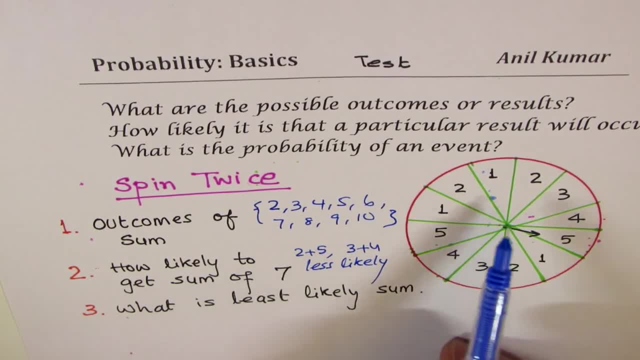 what is least likely now? you will notice that we have numbers 1 to 5, 1 to 5 and only 1 and 2, so these two are there. so what is least likely now? if you look for combinations 1, 1 is least likely. 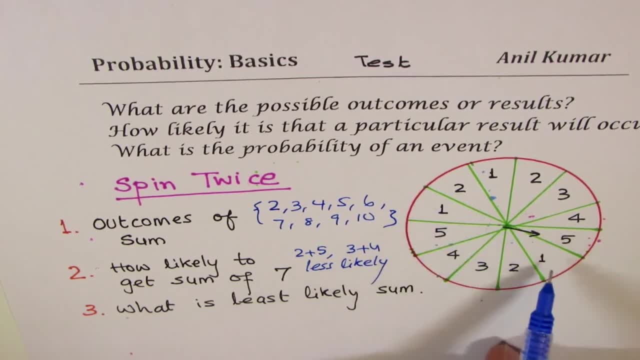 do you see that? because sum of 2. so the least likely is sum of 2. you could say sum of 5 also. there are three ones, correct, sum of 5 and 5 is 10. so least likely should not be sum of 2 but sum of. 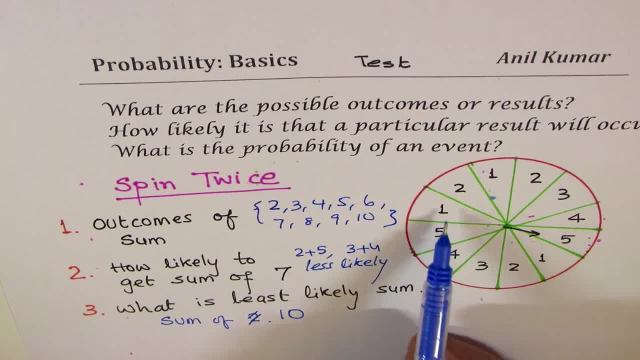 10, since we have three ones, so you can get more time ones but less time fives. there are only two fives here, so the least likely will be the sum of 10, do you understand? so that is a kind of tricky part. so sometimes you know you may get a wrong answer for this, but look. 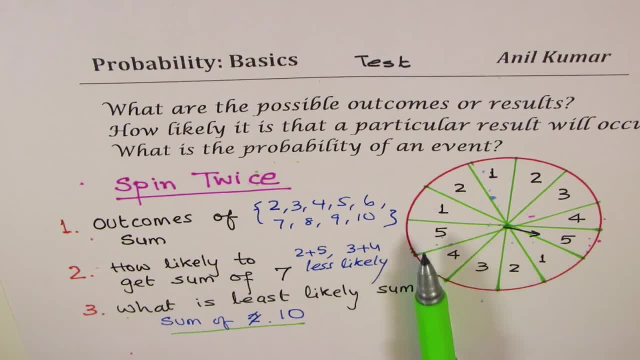 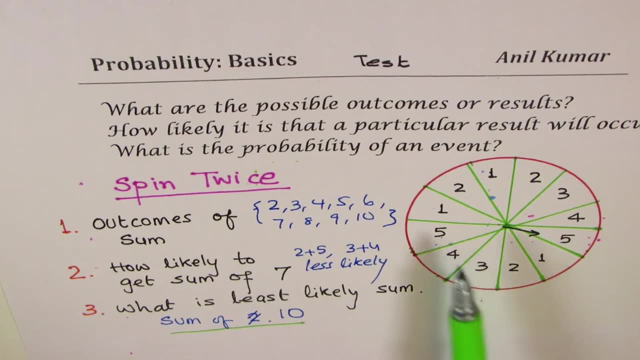 here you got only one combination of making 10, that is, adding 5s, and there are only two 5s. there is only one commission to make two, but there are three ones, so that makes it more likely than 10. you get my point. so with this I 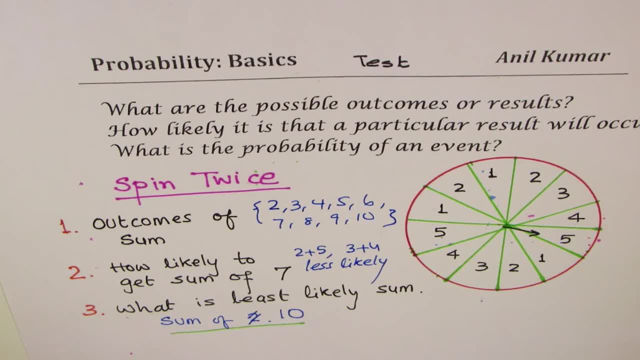 hope you understand how to find outcomes and likelihood of an event when a spinner is given to us. feel free to write your comments, share your views and, if you like, and subscribe, that'd be great for me. thank you and all the best. 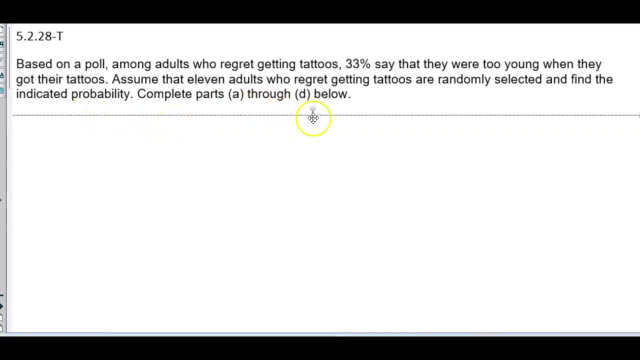 Based on a poll among adults who regret getting tattoos, 33 percent say that they were too young when they got their tattoos. Assume that 11 adults who regret getting tattoos are randomly selected and find the indicated probability, We're going to complete parts a through d below. 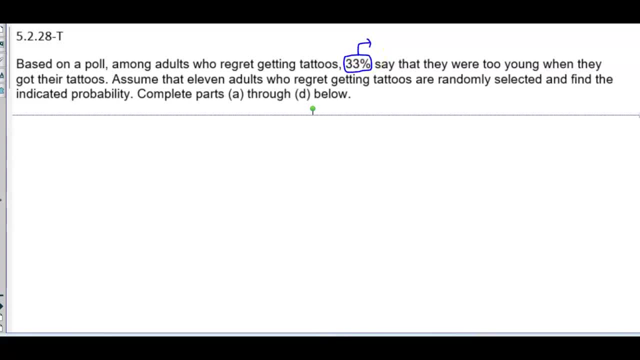 Now the probability that we're given is 33 percent, so p is going to equal 0.33.. And then how many were randomly selected were 11.. So then that tells us the number of trials is equal to 11.. Now let's go ahead and then answer the question. Find the probability. 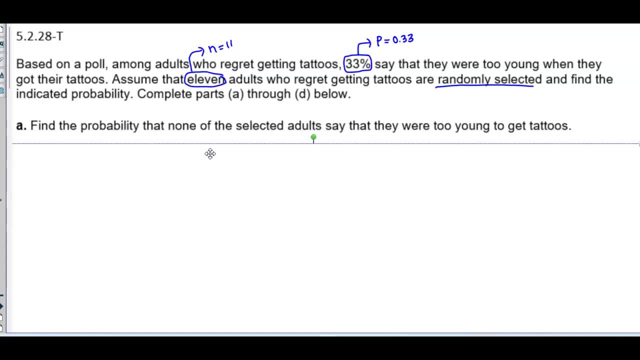 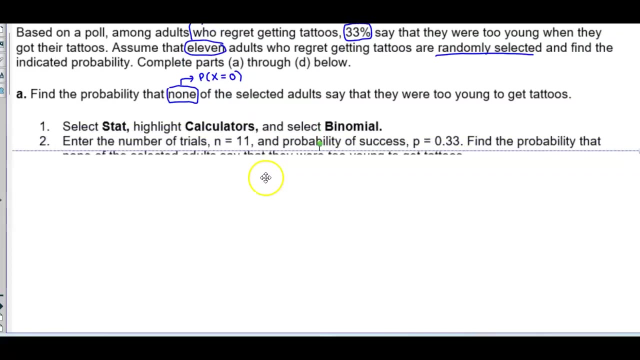 that none of the selected adults say that they were too young to get tattoos. None would mean that you would have zero, so that would tell us that the probability of x would then equal zero. So, using Using StatCrunch, we're going to select Stat, highlight Calculators and then select Binomial. 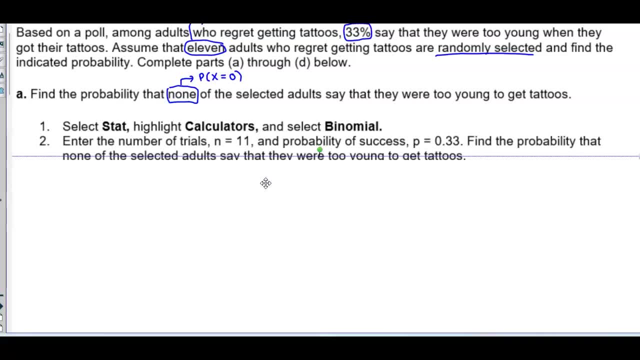 We're going to enter the number of trials, where n is equal to 11, and the probability of success is p is equal to 0.33.. And then we're going to find the probability that none of the selected adults say that they were too young to get tattoos. 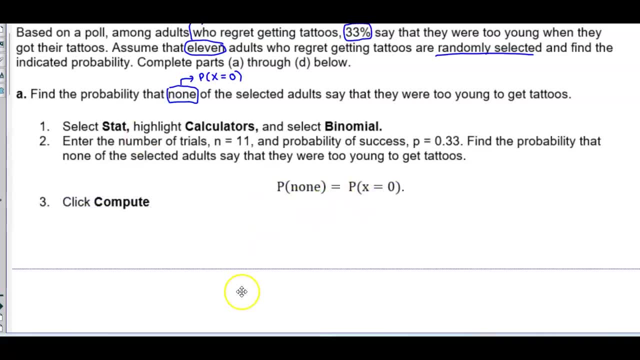 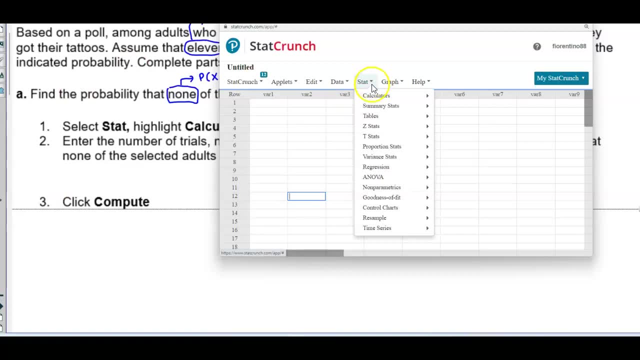 So the probability of none is equal to the probability of x being equal to zero. and then we're going to click Compute, So opening up in the StatCrunch. we're going to select here Stat Calculators and then go to Binomial.